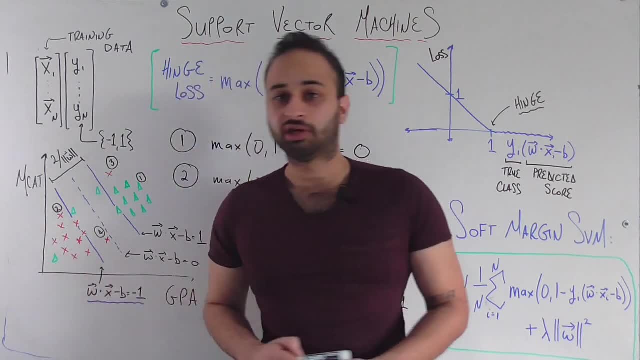 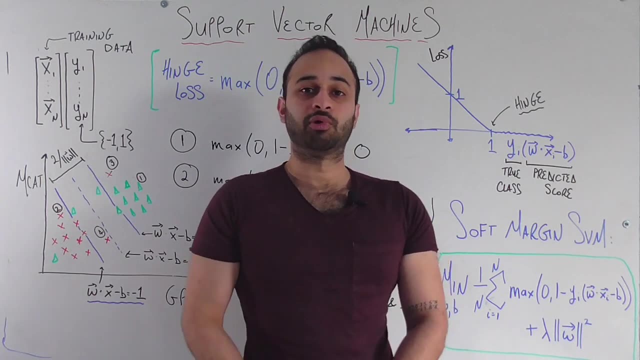 who have low GPAs and MCATs, such as this small triangle down here, but they do get in because of the other factors we were talking about. So this is the real world. this is messy. we still want to use SVM, but we cannot use the. 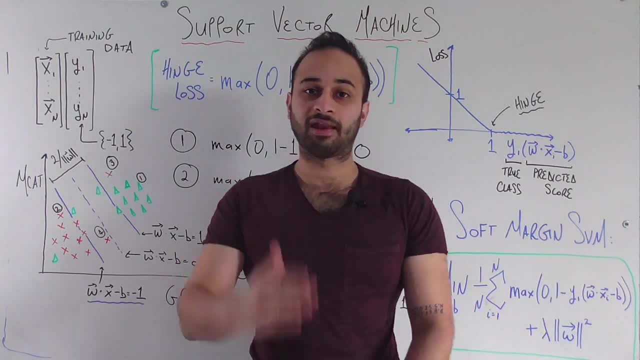 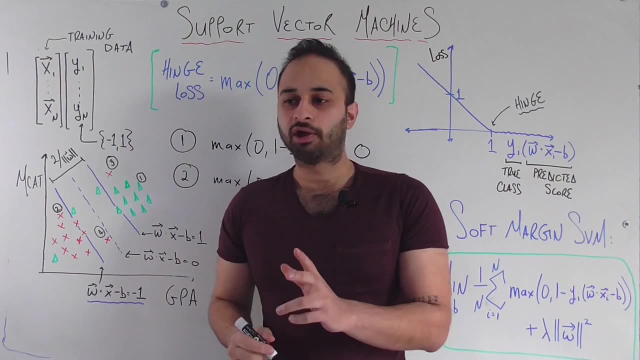 hard margin, SVM, because it just doesn't know what to do when we can't achieve a clean linear separability, Which is the case here. so we need to make our margins a little bit more fuzzy. we need to say that. okay, I want you to classify things as well as possible, but I need to be willing. 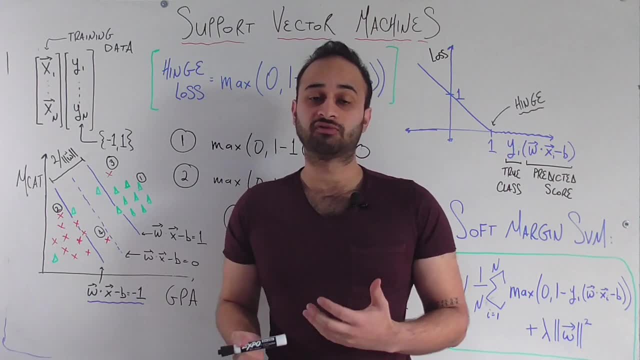 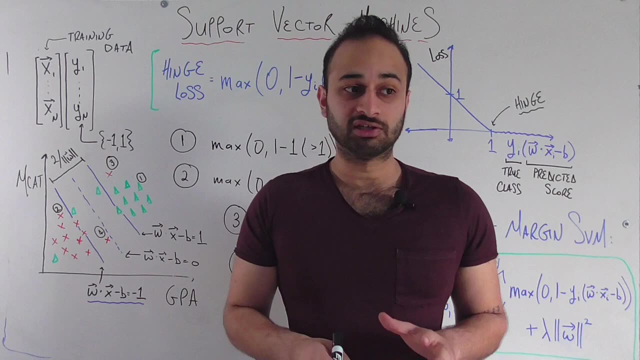 to accept a certain level of mistakes, but I'm going to give you certain penalties for mistakes based on how big they are, and that is the spirit of soft margin SVM. So the quantity that is the driving force behind soft margin SVM is the hinge loss. and 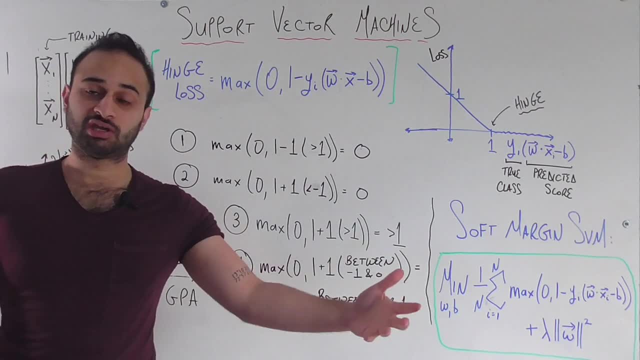 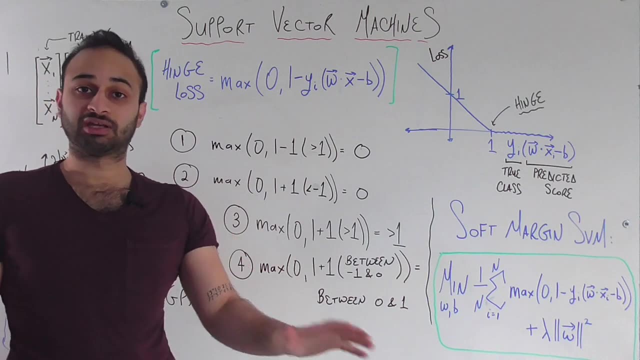 the hinge loss is one of the types of loss I covered in my loss functions video, which I'll link below, But it basically looks like this: looks like a scary mess equation, but I'm going to break it down for you, So let's label the various parts of this equation to get a better idea of the story that it's. 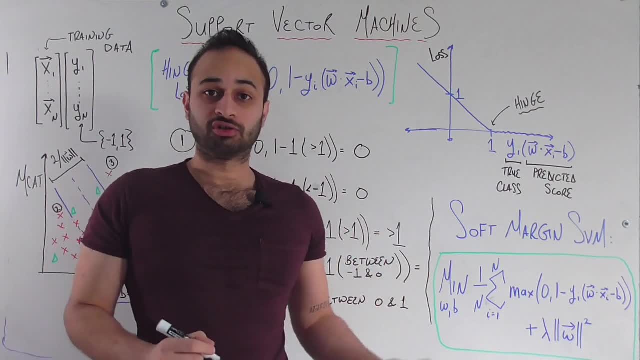 trying to tell us and why it's doing the job we want it to do. Yi, again, is the true class of the student. so this is one or negative one. This other quantity is the score that we're giving to the student. so I'm going to call. 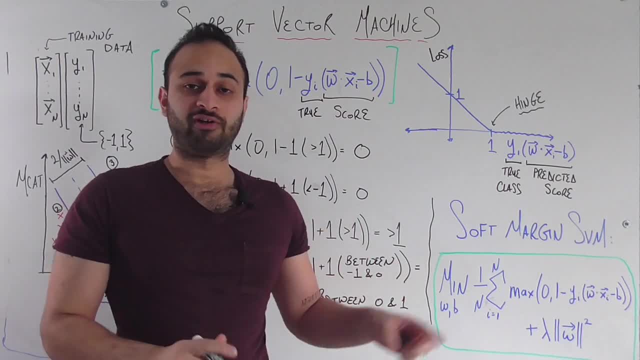 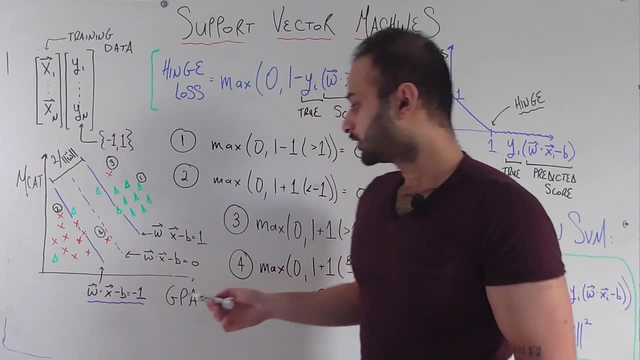 it score, but I'll explain exactly what it means. So this quantity is w, our vector of weights, times xi, which is the predictor for any given student, minus b, which is our intercept. Now, if we look at the three lines here, as we said in the last video, they each have different. 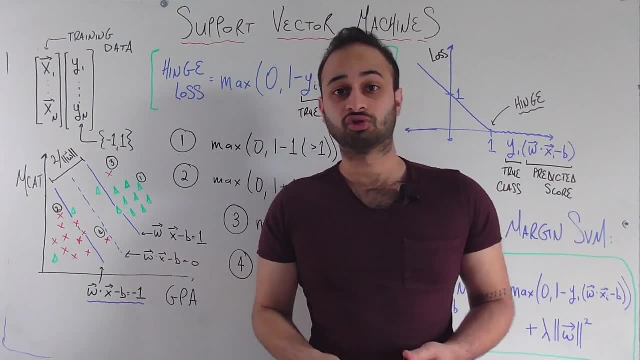 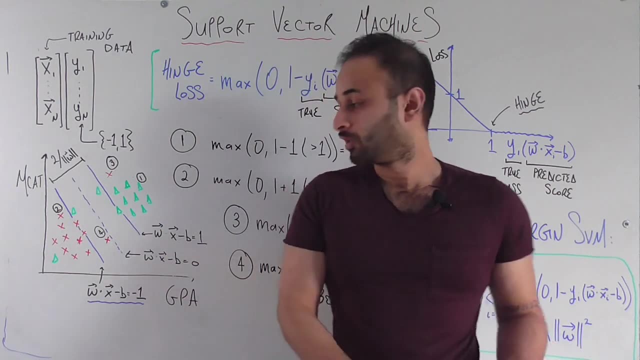 equations. The top line is: w dot x minus b is equal to one. The decision boundary is that quantity equals zero and the lower line is that quantity is equal to negative one. Notice that that quantity, which is w dot x minus b, is exactly the quantity that I've 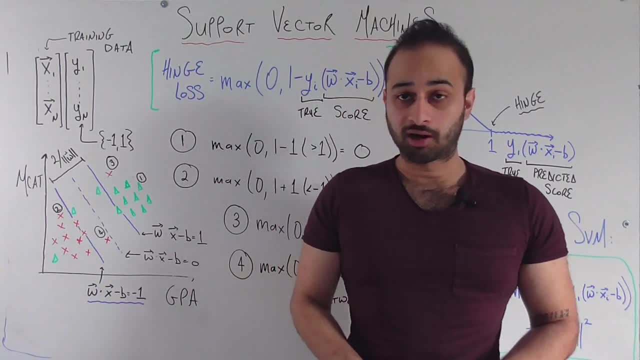 written right here, which I've called score. The reason I'm calling it a score is because anything that is on this side of this top blue line has that score or that quantity greater than one. So if we look at the three lines here, as we said in the last video, they each have different. 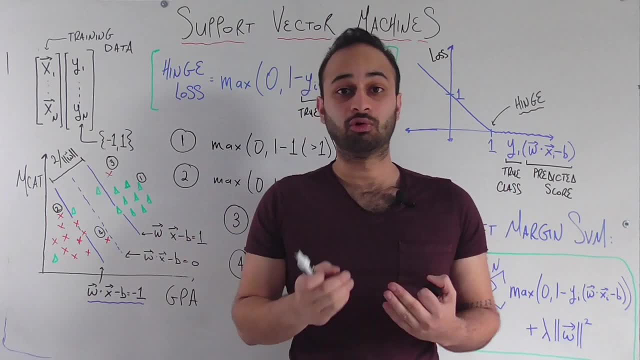 equations. In the last video we said that a score equal to negative one had that quantity greater than one. so if we look at the drawing here, we have that this line is where that score would be equal to one. so anywhere above that line it would be greater than one. 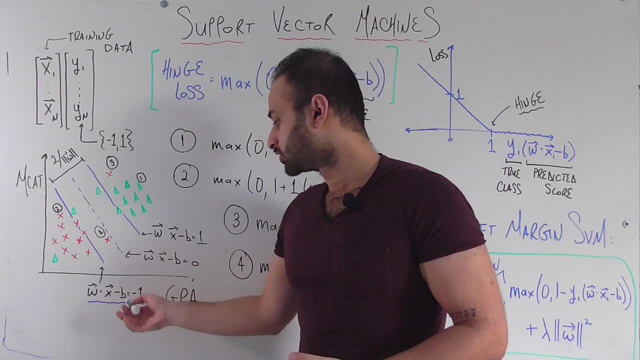 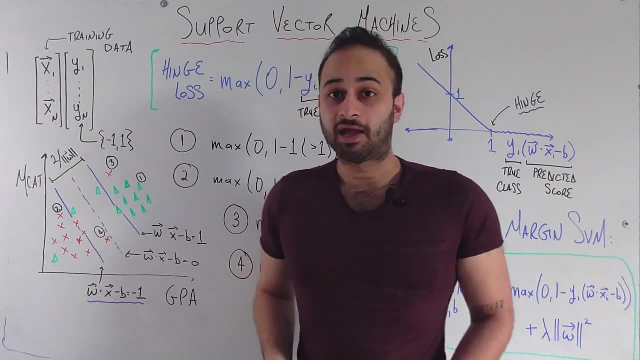 Now, with the same logic, we can say that this bottom line is where that score is equal to negative one. So any observation we see who is below that line is going to get a score that is less than negative one, and anyone who is within the margin. so which is below this top blue? 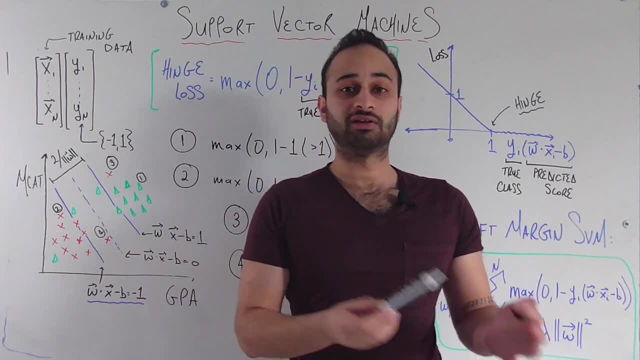 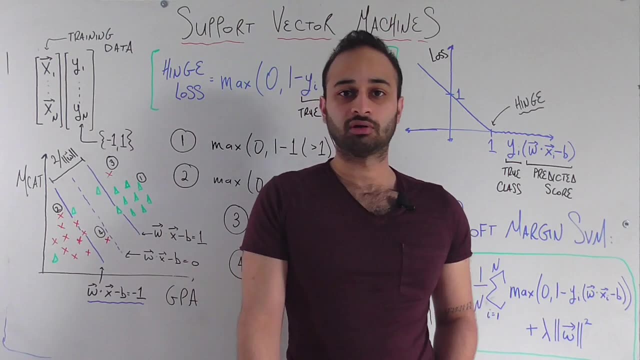 line, but above this bottom blue line is going to get a score between negative one and one. So it's going to be between zero and one for this region, and it's going to be between zero and negative one for this region. Now, why is this important? Why do we need to introduce this? 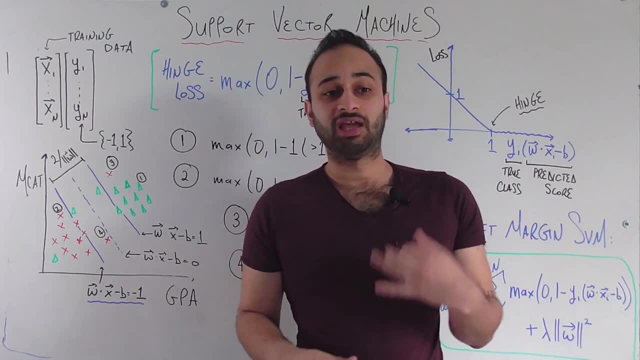 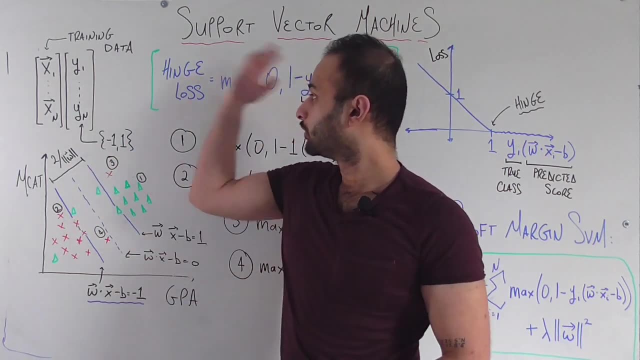 concept of score to continue telling our story, Because we want the classifier to behave in a certain way. We want it to say that any observation which is very far away from this top line- so who is all the way over here, let's say- gets confidently predicted as a positive one. So for that observation, 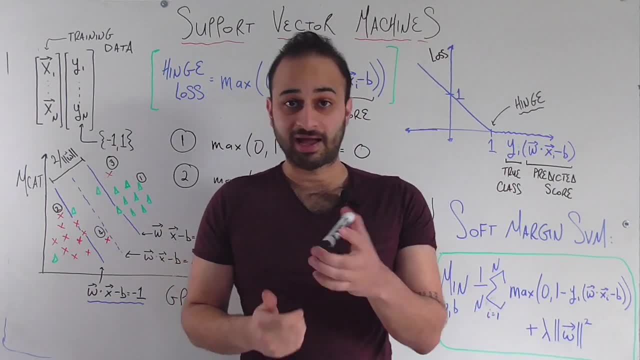 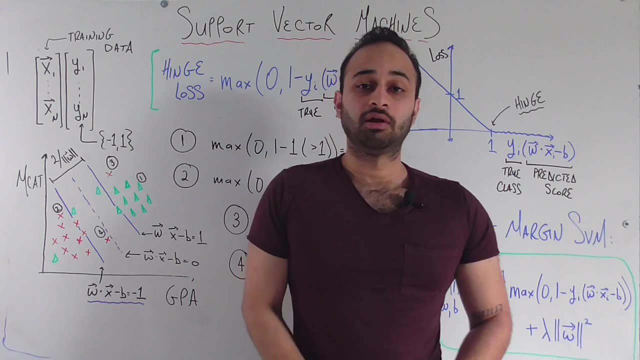 the score will be very, very positive. So we better have that. the class of that observation is actually positive as well. On the other hand of the story, we have that if there's an observation way down here, the score of that student would be very negative. so much less than negative one. So we 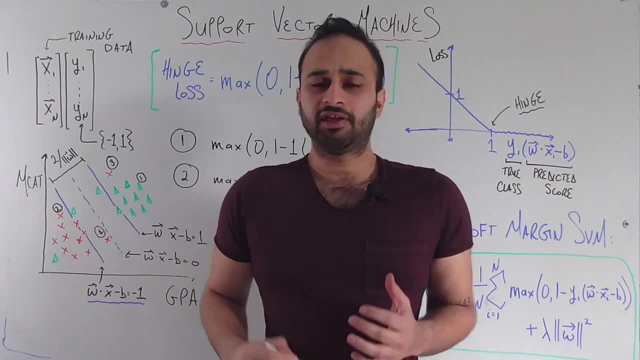 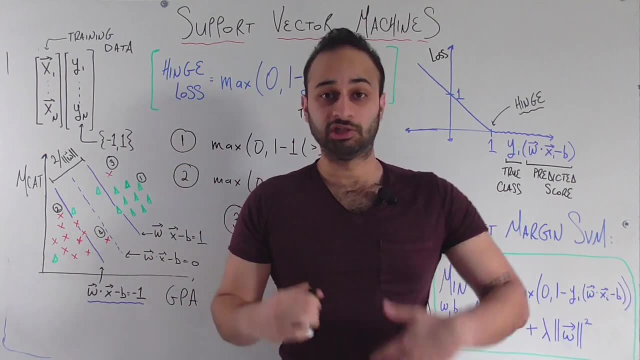 better have that. the truth about that observation is negative one, And so I think it's even easier to get a sense of this hinge loss by just looking at the couple of observations that I've labeled here and see what the hinge loss comes out to for each of those observations. So let's look at these. 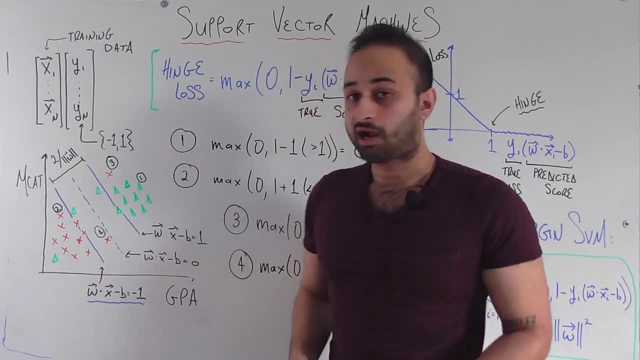 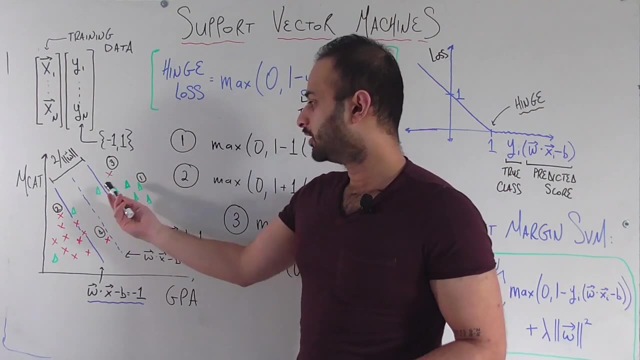 four observations. The first one is this green triangle. Now, we're generally happy about this green triangle- if this is our classifier Here- because it is well inside the region, that is, above this blue line, and it is truly a student who does get into their top choice medical school. So let's work out the math a little bit. So for 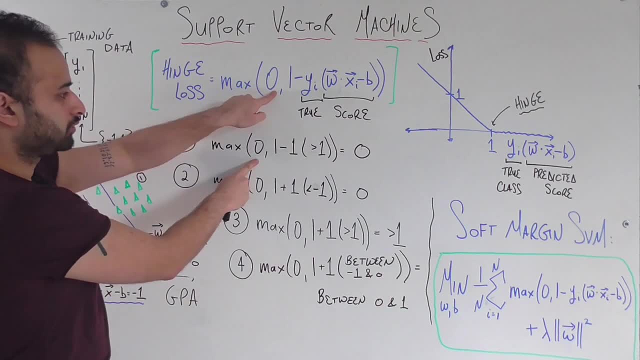 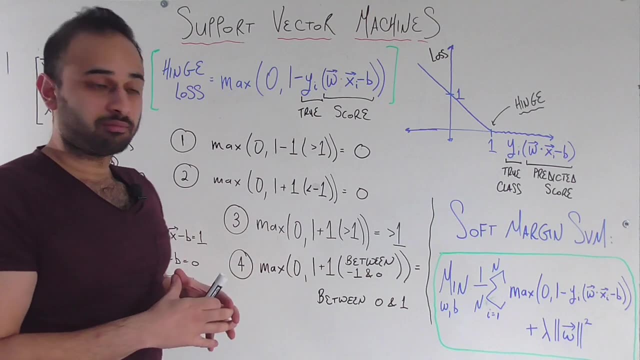 this student. so for student one it's going to be max of zero, one minus, and their true class is equal to one. And what is their score going to be? Their score is going to be above one because they are above this blue solid line here. So if you work out the math here, this comes out to zero. 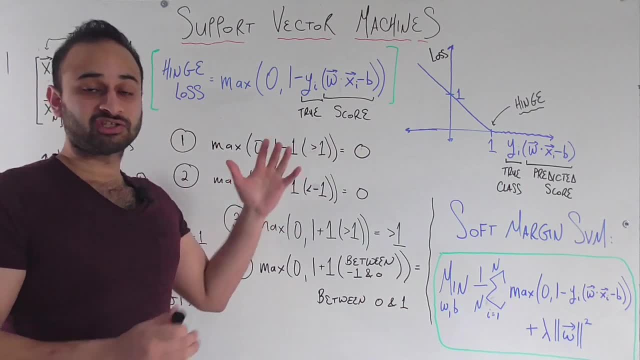 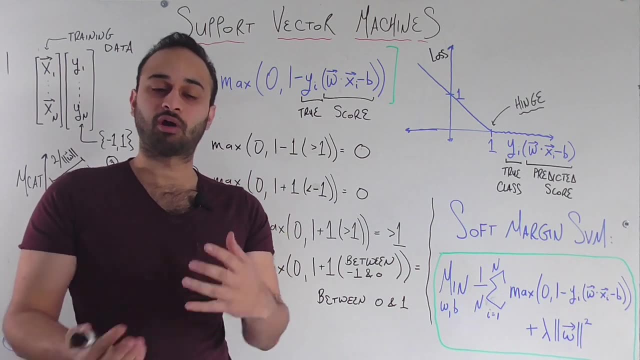 because the second term is negative, therefore max of zero and a negative number is zero, And so we're saying the loss for that student is zero, which means that we are happy with that and we're not assigning it any loss. So far, so good. Let's look at the next. 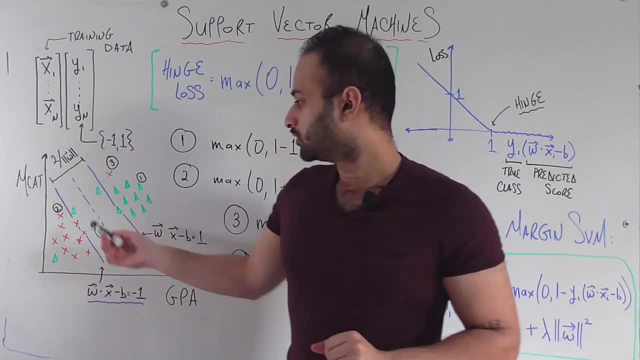 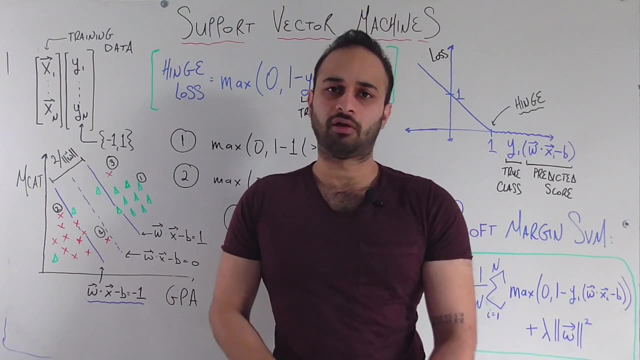 student in our set. Let's take a look at student number two. Student number two is basically the opposite story. So they are below this lower blue line and we're also happy about that because they're on the correct side of the margin. They're on the negative one side of the margin. Let's see. 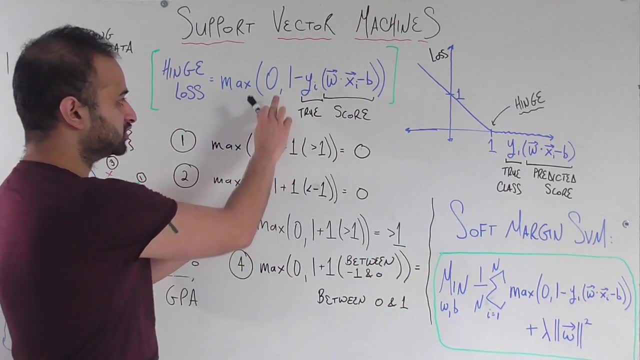 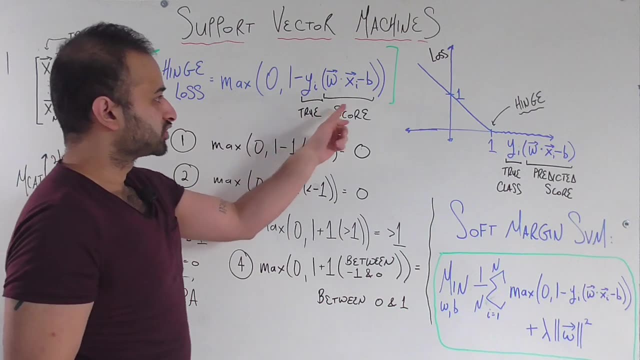 what their hinge loss comes out to. So their hinge loss comes out to max of zero one. their yi is equal to negative one. so this sign flips to a plus and this score is going to be less than negative one based on the story that we just told. So we put a less than negative one here. 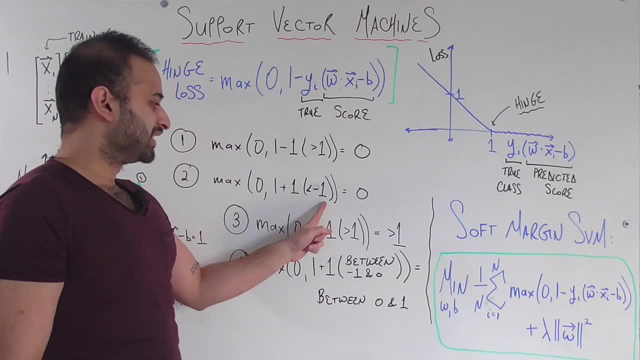 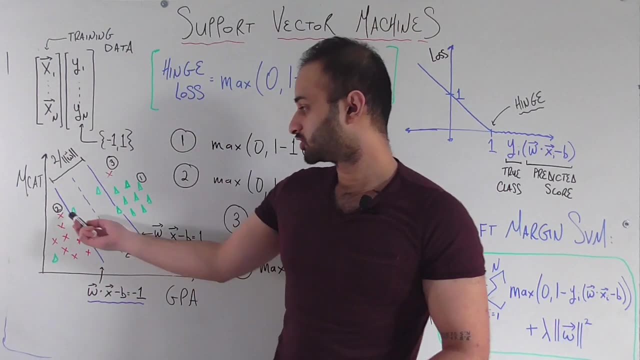 and if you work out this math, this quantity also will be less than zero. therefore, the max is going to be zero, which again makes sense, because we would like to assign a loss of zero to person number two, because we're happy about the way the classifier is performing on them. So no loss there. 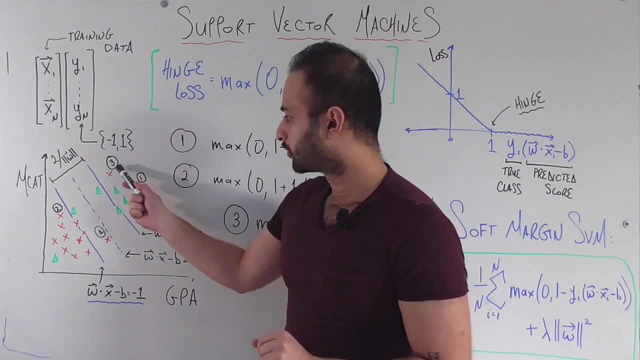 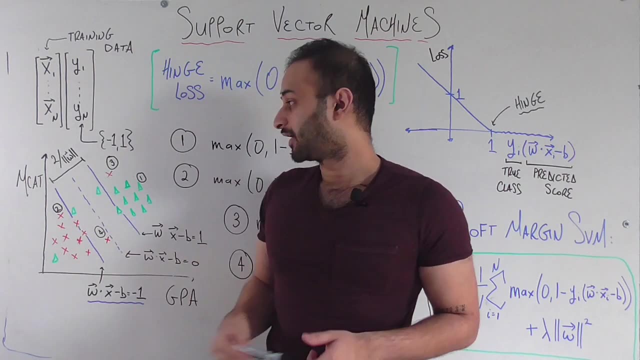 Here's where the story gets more interesting. So let's look at observation number three. so this is a student who does not get into their top choice medical school, but based on the classifier that we currently are looking at, they are categorized on the wrong side of the margin, so we would like their loss to be high. 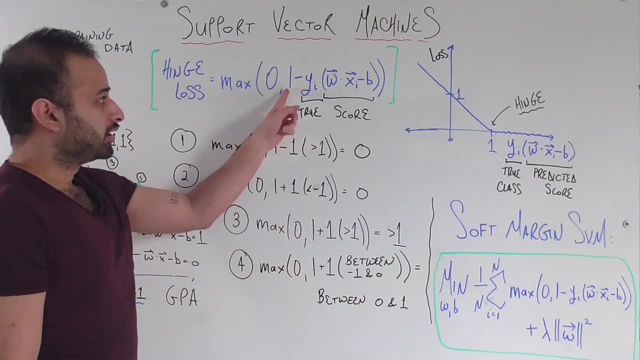 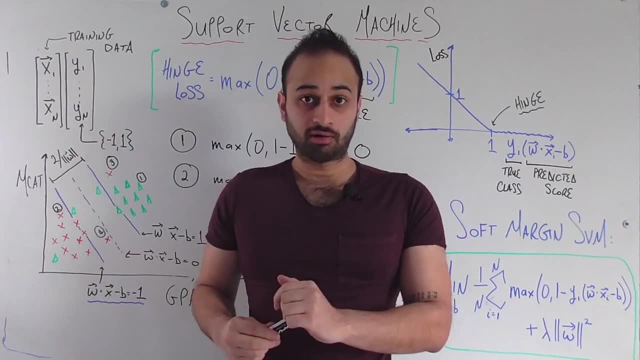 Let's see what happens. So we're going to have max of zero. one minus their yi is equal to negative one, so the sign flips to a plus, but their score is going to be greater than one because, based on the classifier I'm looking at, they are on this side of the margin. therefore, I have a greater than one here. 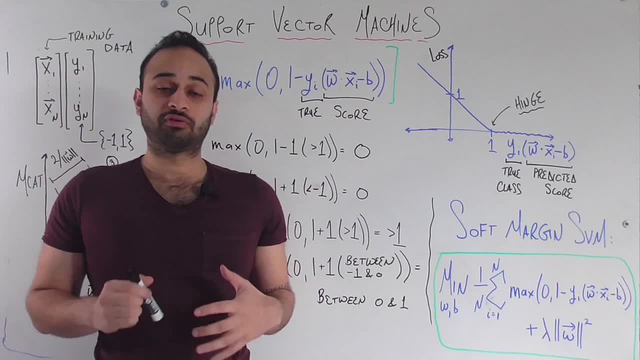 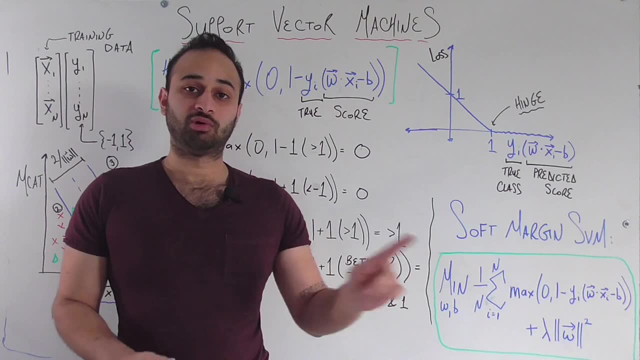 here, this is going to be greater than one. Therefore, this is telling the story that for that person, I'm assigning a loss that is greater than one. I am giving a penalty to the model because it's not doing a good job for that person. And for the last sample, let's look at somebody who 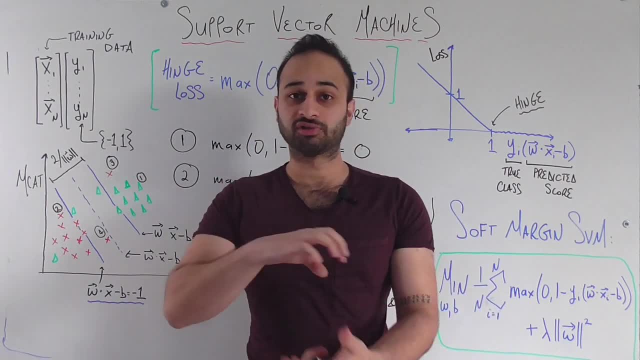 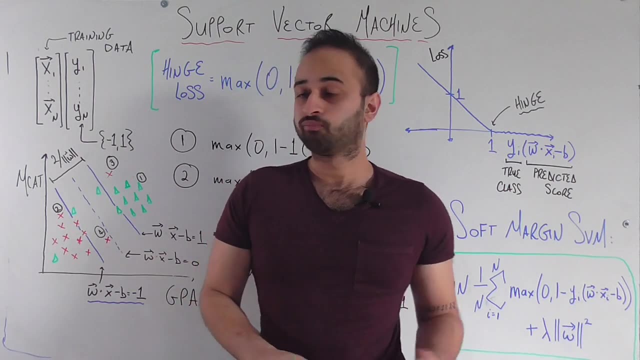 is inside the margin. So with soft SVM we can actually have observations that are inside the margin. So for observation number four, notice that this person actually does get classified correctly, because anyone on the lower side of this dashed line gets classified as negative one, which is what? 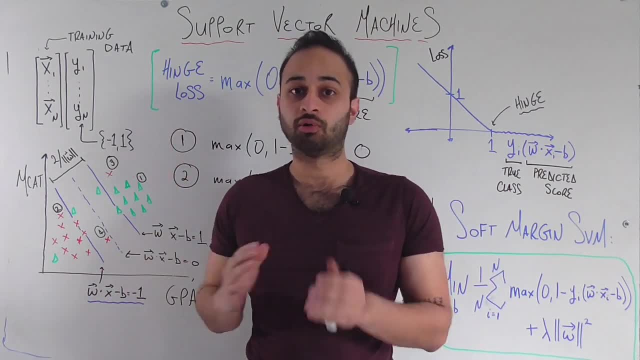 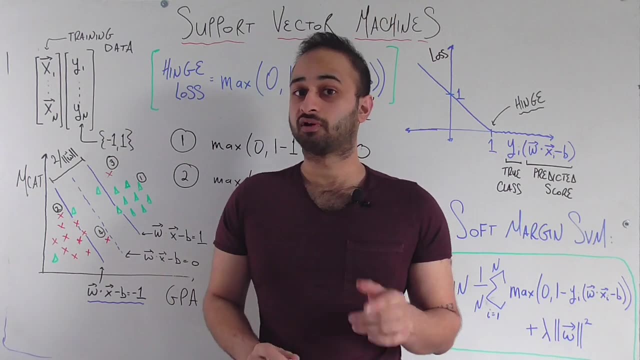 this observation is, and anyone on the other side would get positive one. So this observation is correct, but SVM says that we still want to give it a penalty because it is too close for comfort. It is too close to this dashed line, It is inside the margin, So we want to give it a little bit of. 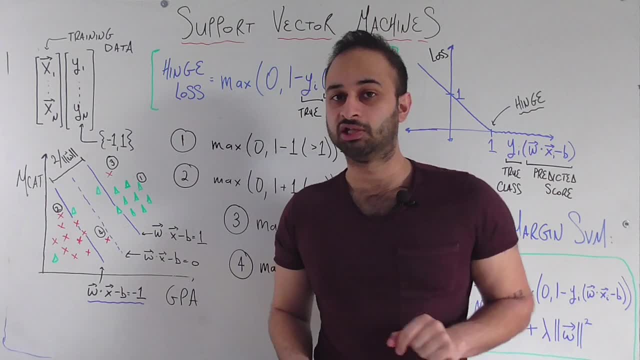 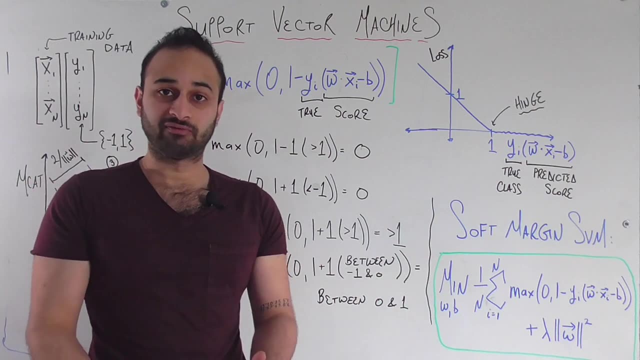 a penalty, but not as big as we did for the previous one. Let's see what the hinge loss does. So for this last one here it's max of zero, One plus and the sign flips again because it's a negative observation. So notice that this score. 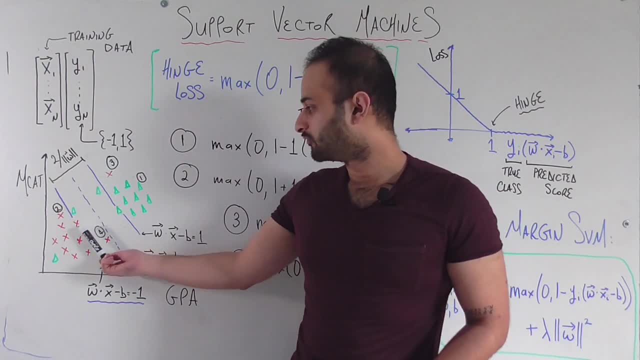 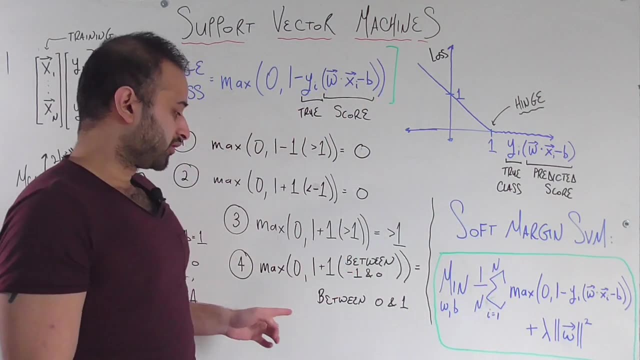 for this guy right here would be something between zero, which is the dashed line, and negative one, which is this bottom line here. So the score is going to be between negative one and zero, which is exactly what we see here. If we work out this math, then the quantity of the hinge loss is: 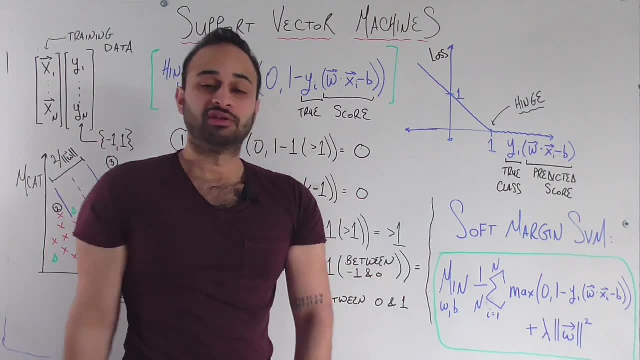 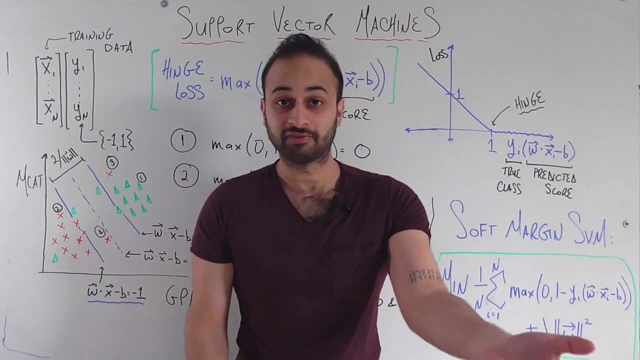 going to be something between zero and one. This is exactly what we want. This is what we want because we're saying that I need to give you some loss because, although I'm classifying you correctly, I'm barely doing that. Therefore, I want to give you a loss between zero and one. 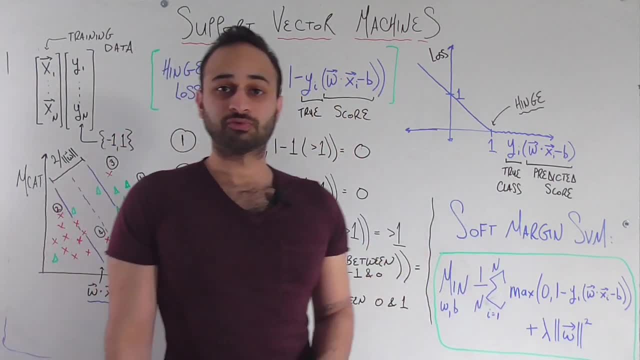 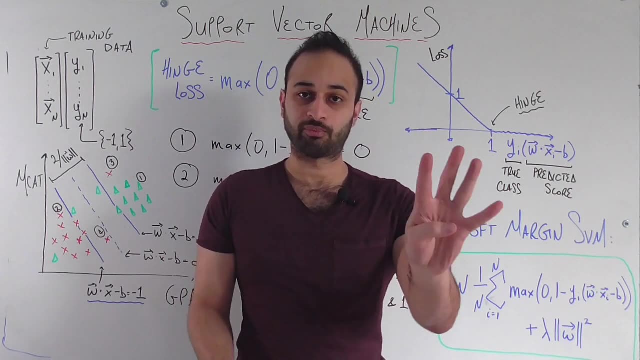 But I don't want to give you a loss that is greater than one, as we did with someone who is clearly misclassified. So that's the story of the hinge loss, told through four examples, And you can come up with more examples here and try to go through this exercise further for yourself. 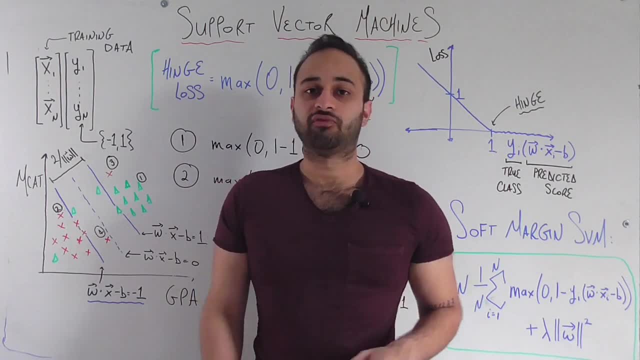 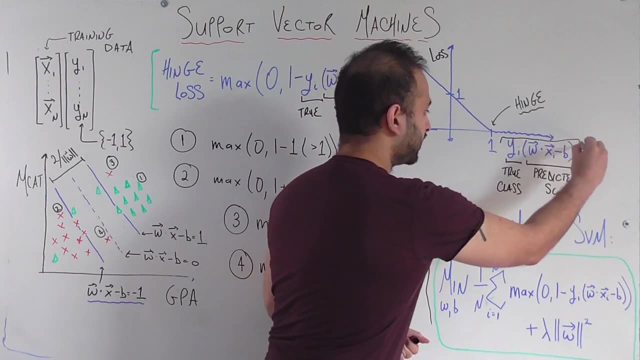 Let me show you a graphical depiction of the hinge loss. Maybe that's going to help you out if you're still having a little bit of trouble grasping it. So I've plotted the hinge loss here On the x-axis. is this quantity, which we've been calling the score times the true? 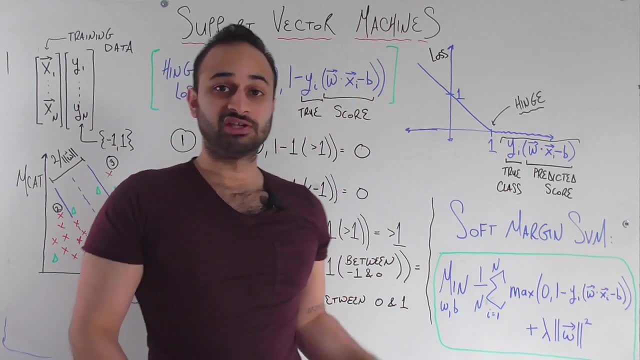 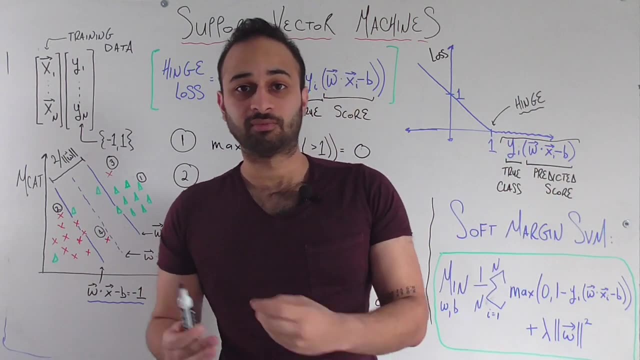 So score times the true and the y-axis is the loss itself. So notice that any time this multiplication works out to something greater than one, that means that that's somebody who is on the correct side of the margin. so we want to give them. 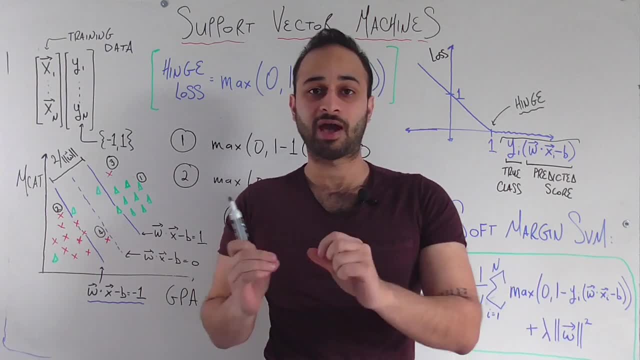 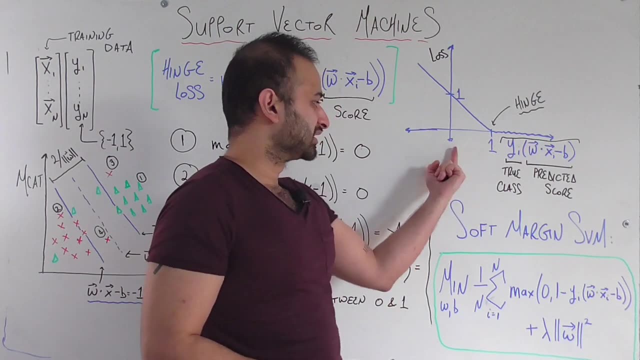 a loss of zero. They are not problematic. we don't want to give a penalty to our model for those people, So that's why the loss is exactly zero for those people, Now anyone for whom this quantity is less than zero, so anyone on this left side of 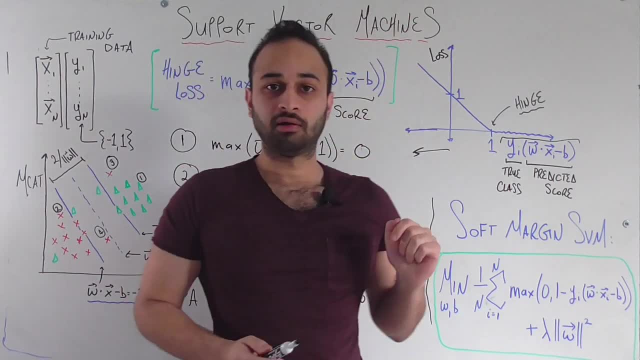 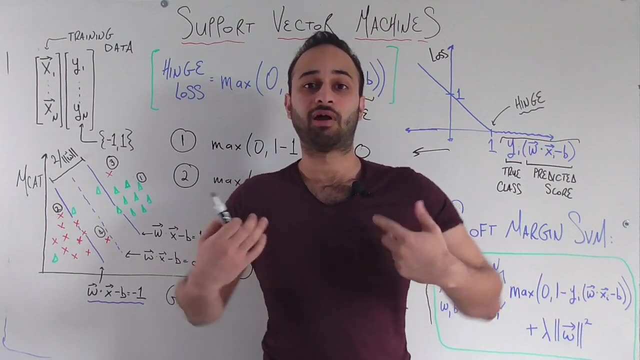 zero is going to have a loss that is greater than one. That's exactly what we saw for case number three here. These are people who are just straight up on the wrong side of the margin, so we want to give a rather big penalty to these people. 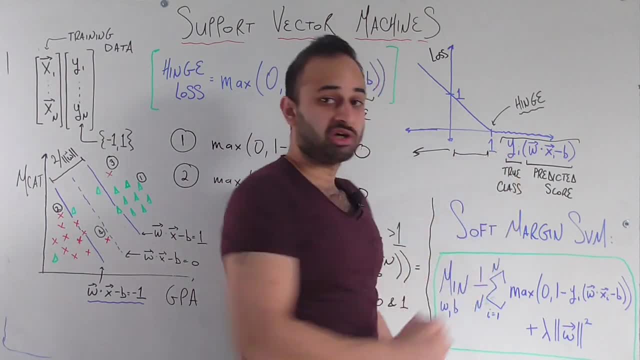 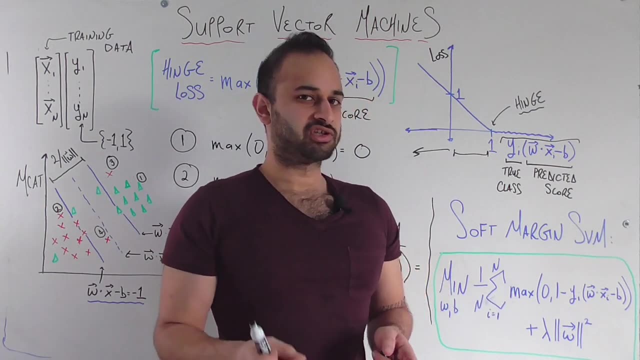 The interesting part of the hinge loss, I think, is the people who are between zero and one. So if your multiplication of these two things is between zero and one, that means that actually you are on the right side of the decision boundary but you're inside the margin. 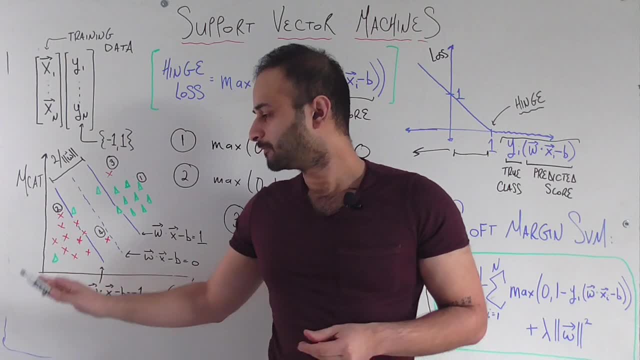 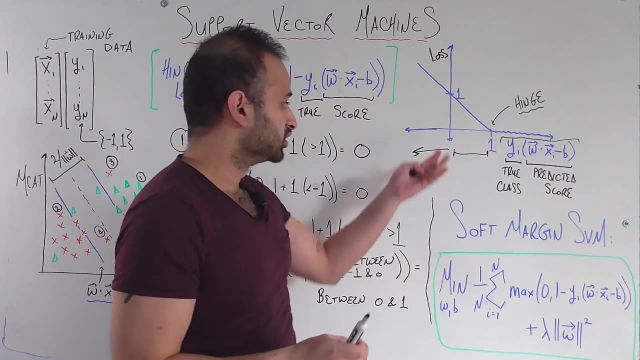 So you're on the right side of the decision boundary, but you are inside the margin. Therefore, we're going to still give you a little bit of a loss, because we're not too comfortable with that situation. So we're going to get a loss between zero and one. 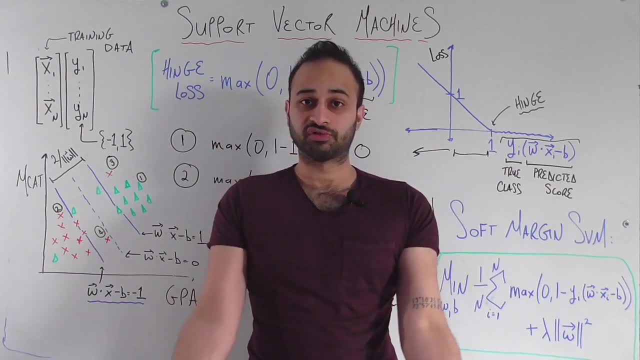 So that's the story that hinge loss is trying to tell. That was the hardest part of this video- was just kind of getting an intuition about why this quantity of hinge loss is so crucial to our soft margin SVM. The final thing we'll look at in this video is the equation, the mathematical formulation. 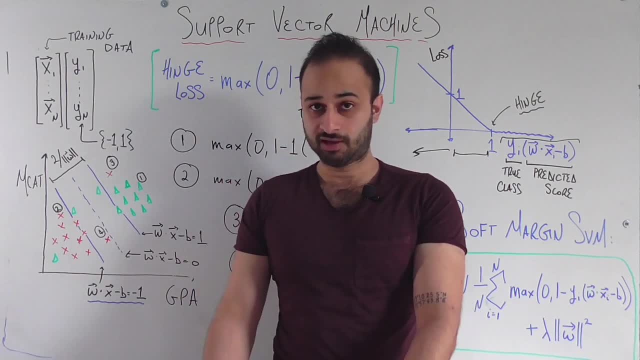 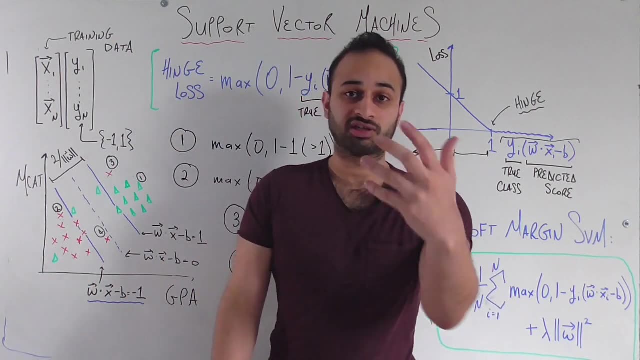 for the model of soft margin SVM. Soft margin SVM is given by minimizing the following quantity: So I want to pick a- w and a- b. I want to pick a vector of weights w and an intercept b, such that I'm minimizing the sum of these two terms. 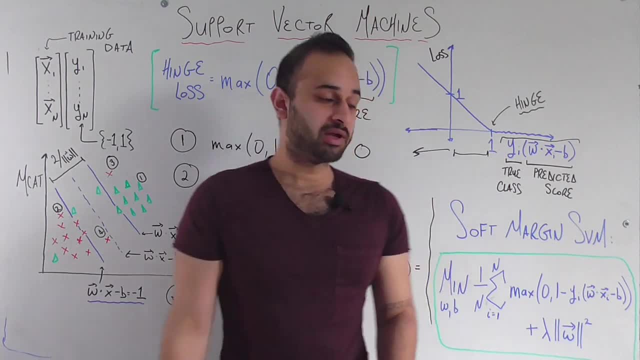 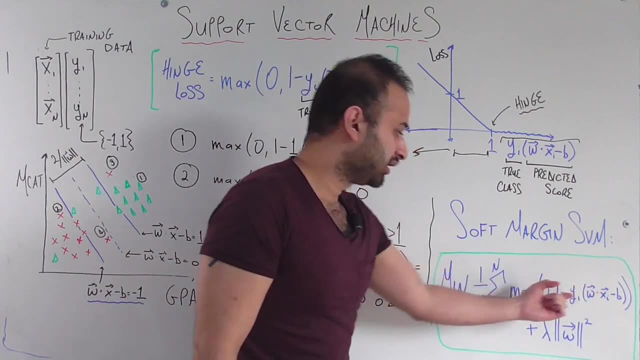 And these two terms tell the exact story we want to tell. The first term is summing over all of our observations from one to n. so everybody who's in our training set- And the thing you're looking at in here is literally just me- copying the hinge loss formula. 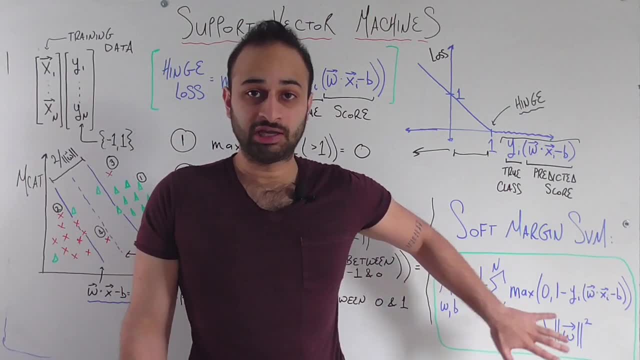 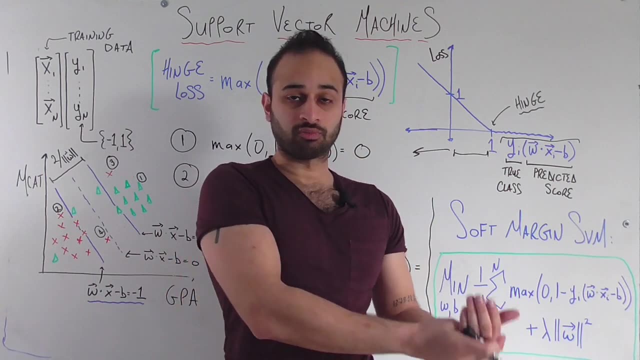 here And then we divide by n. So this is the average hinge loss of a classifier across the entire training set. Of course We want that to be as small as possible. We want as small of a hinge loss across the entire training set as we can get. 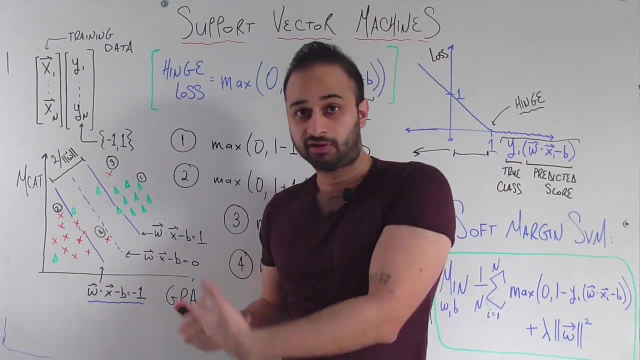 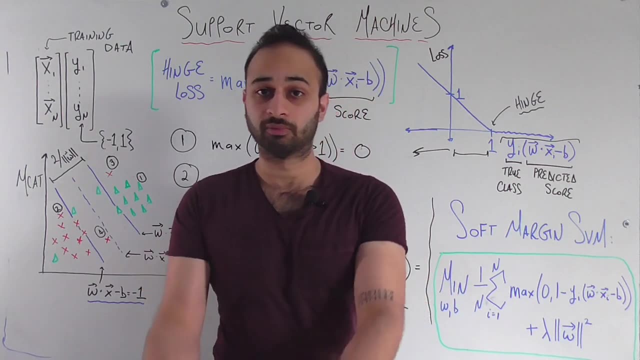 But that's not the end of the story. We also want to, in the spirit of SVM, to maximize the margin which, as we saw in the previous video, is analogous to minimizing the magnitude of w. So we also want to add a plus lambda times the magnitude of w squared here, so that we 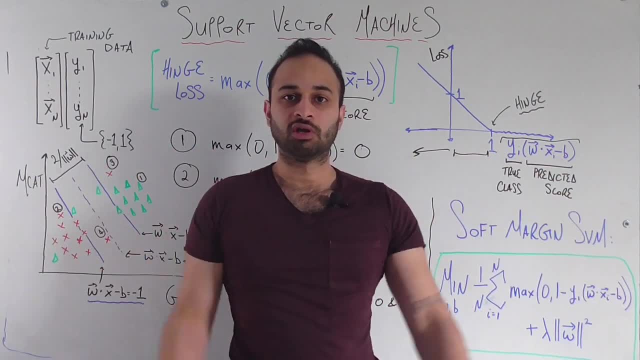 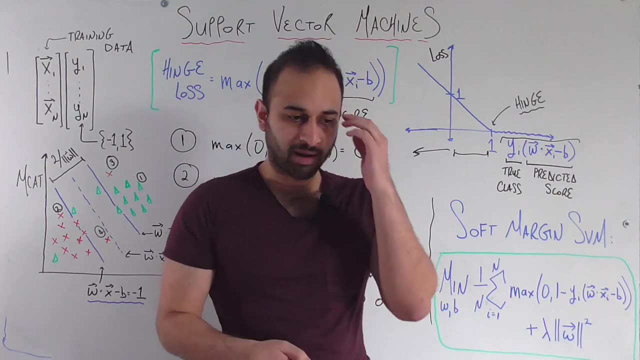 can also work on maximizing the size of this margin. So this formula, Although It's going to be confusing, it's telling a very interesting story. It's saying that I'm trying to do two things simultaneously when I have real world data. 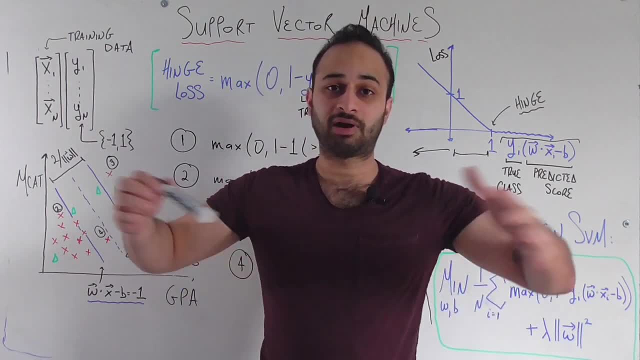 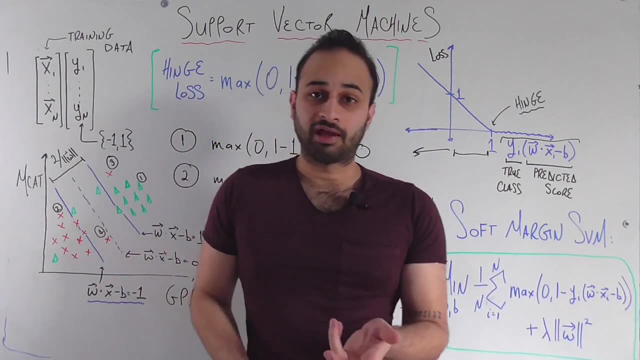 The first thing I want to do in the spirit of SVM is to maximize the margin. I want to maximize the separability between the two classes, And that's what you're seeing in the second term here, But I know that in real world I'm going to have a little bit of misclassification. 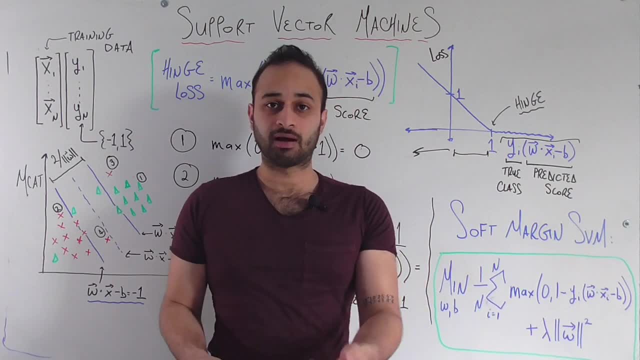 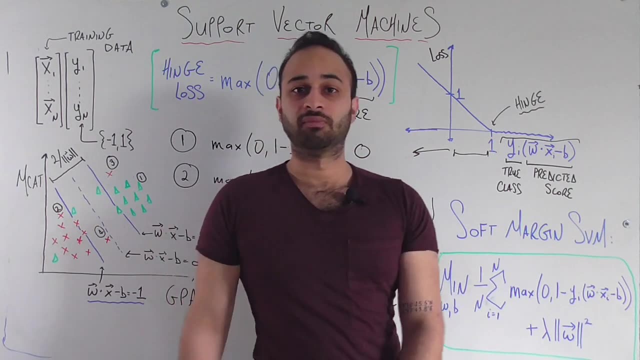 So this first term is basically saying that I want the loss that comes from that misclassification to be kept in check, To be as small as possible. So that's what's going on with this minimization sum you're seeing here, And the last thing I'll say is: what is this parameter lambda?